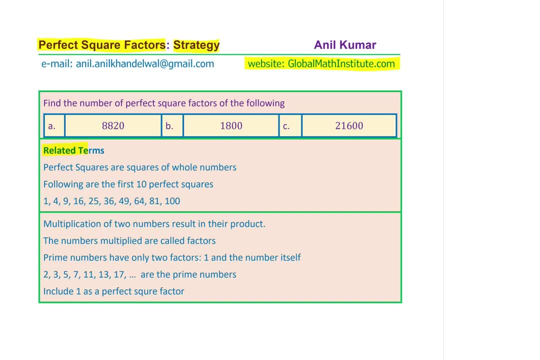 Well, let's look into the related terms, as these terms may be new for some of you. What are perfect square factors? Well, the perfect squares are squares of whole numbers. For example, following are the first 10 perfect squares: 1 square is 1, 2 square is 4, 3 square is 9, 4 square is 16, 5 square is 25,. then we have 36,, 49,, 64,, 80,, 100 as squares of 6,, 7,, 8,, 9 and 10.. 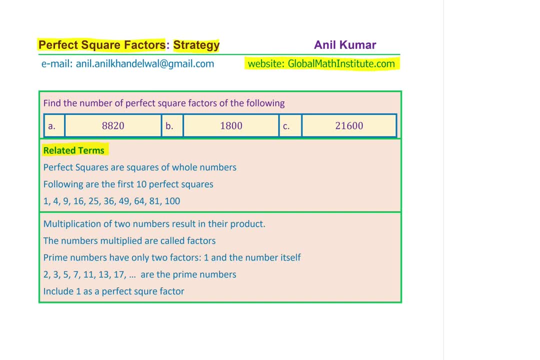 So, likewise, we have squares of every number, which are called perfect squares. So n squared, So n squared will be a perfect square where n belongs to the set of natural numbers, correct? So that is the whole idea. Now, what are factors and how do we relate perfect squares and the factors and answer the question? That's the second part of this. 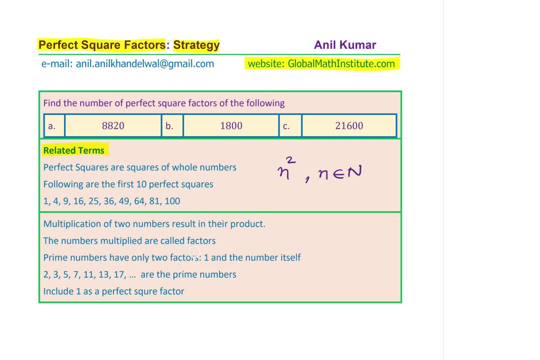 As you know, the numbers, when multiplied, are called factors. For example, if I write 7 times 6 as equals to 42,, in that case 7 and 6 are factors of 42. Right, So that is what factors are. 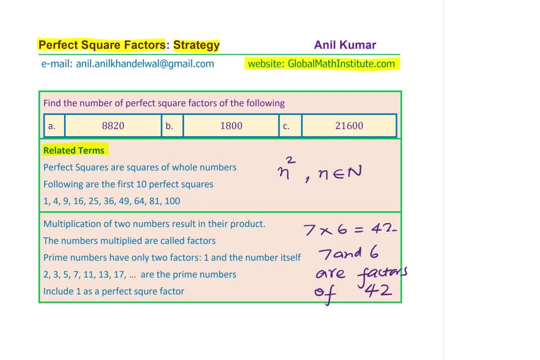 So 7 and 6 are factors of 42, and 42 is the product of 7 and 6.. So, basically, the numbers multiplied are called factors and the prime factors. what are they? Well, the prime numbers have only two factors, which is 1 and the number itself. 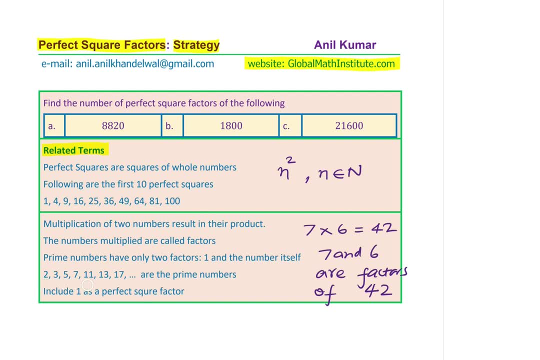 The examples of prime numbers are 2,, 3,, 5,, 7,, 11,, 13,, 17 and so on. So all these numbers have only two factors: 1 and the number itself. Note that 1 is not a prime number, since 1 has only 1 factor. 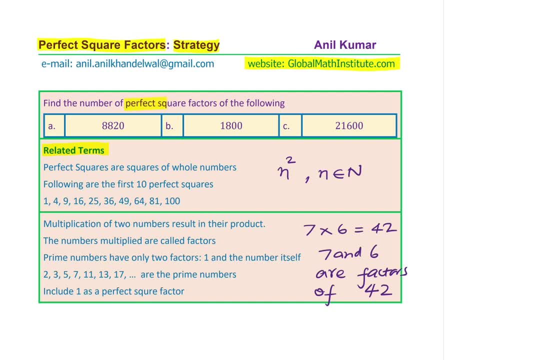 However, when we are talking about perfect squares, in that case 1 should be included as a factor, the perfect square as you have seen here right now. keeping that in mind, let us see how to find the number of perfect squares of the following. we'll begin. 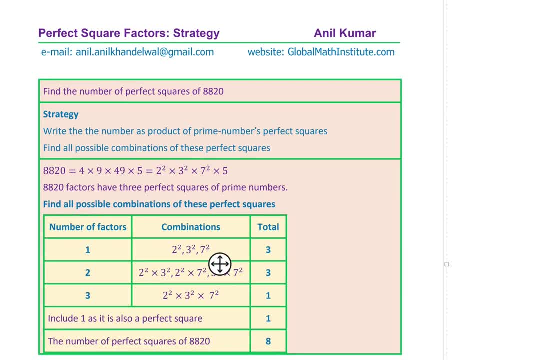 with 88- 20. now let us see the strategy to find the number of perfect squares for 88- 20. the strategy is: write the numbers as product of prime numbers, perfect squares. you get the idea. prime numbers, perfect square, like 2 square, 3 square, and so on. find all possible combinations of these perfect squares. 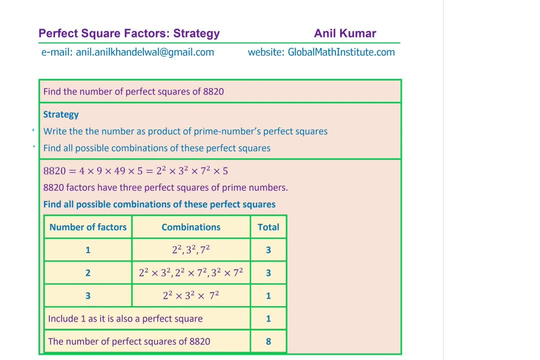 so these are two steps which will follow to get our solution. for example, 88, 20 can be written as 4 times 9 times 49 times 5, that is, 2 square times 3 square times 7 square and 5 square. well, how do we get these numbers? let's look into. 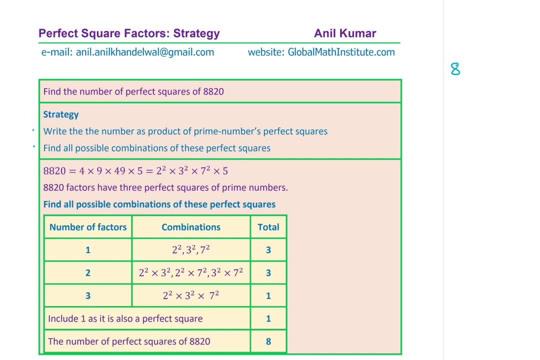 this process so we can do like this: let's take the number 88, 20 right, so we can get do the prime factorization of this in a way that will divide this by the square of the prime numbers. for example, this is an even number which can be divided by 4. 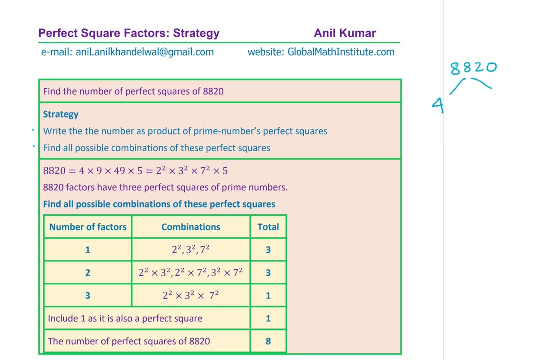 correct. so if I divide by 4, what do I get? I get 2, 2 0, 5, good ending with 5, correct. so if I divide by 4, what do I get? I get 2, 2 0, 5, good ending with 5. 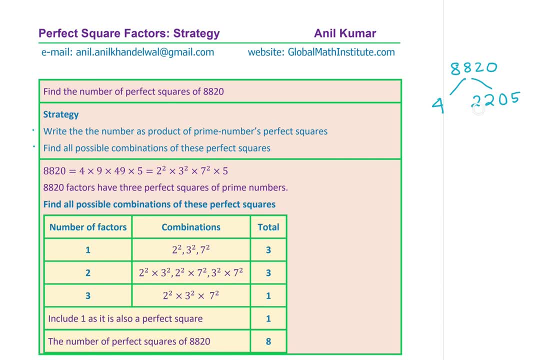 right. and also sum is what: 2 plus 2 is 4, 4 plus 5 is 9. that means I can also divide this by 9, so let me now divide this by 9, so 9. when dividing 2, 20, 5, 9. 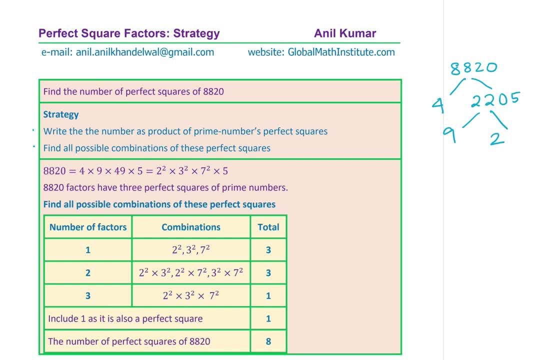 times 2 is 18, 40 means 9 times 4 is 36 and 45 is 9 times 5, so we get 245. now 245 can be divided by 2 and 5. what well, you can divide this by 5. I know 5 is not a perfect square, but 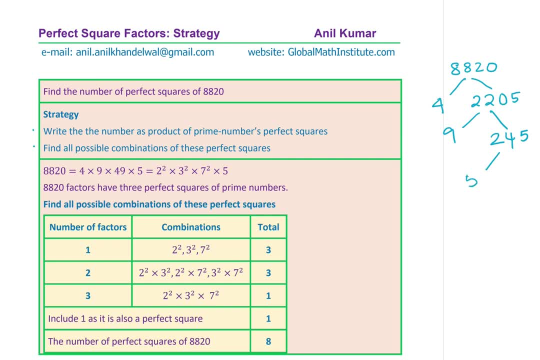 still, let's see what do we get. so if I divide this by 5- I know 5 times 4 is 20 and 5 times 9 is 49- what do you get? see, you get some perfect squares. now, 4 is 2. 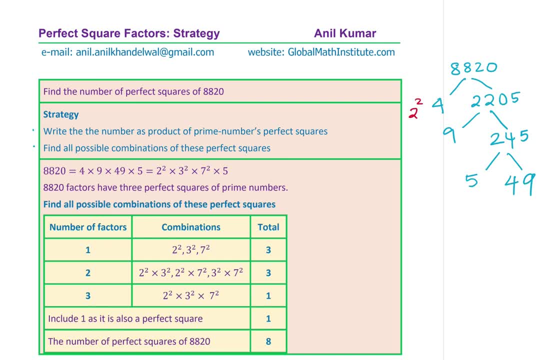 square, correct? so this is like 2 square, 9 is 3 square and 49 is 7 square. so we can now write the number 8820 as the product of 2 square, 3 square, 7 square and 5. you get the idea. so that is how we get this list of the factors which are: 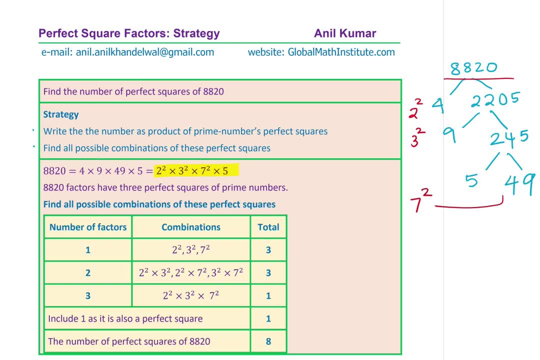 perfect squares. so 2 square 3, square 7, square times 5 is what is we get from the number 8820.. So I hope you understand this process of kind of factoring right. Well, we're trying to divide by the perfect squares to make a job simpler. 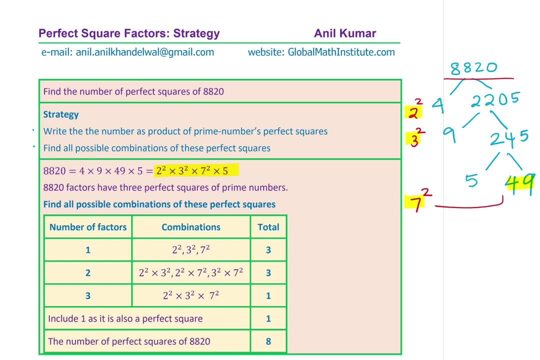 Now we know that these are the perfect squares and factors of 8820.. But remember, their product will also be a perfect square, correct? So that is kind of important to understand, right? So 2 squared times 3 squared is also a perfect square, correct? 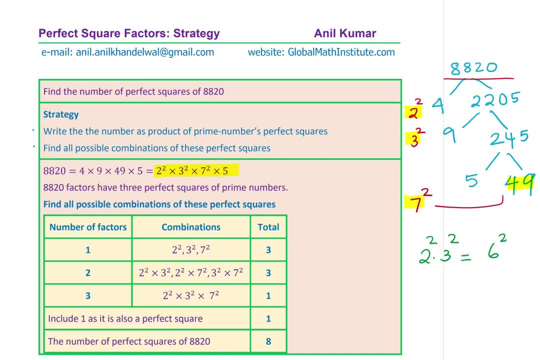 2 times 3 is 6,, which is 6 squared. So 6 squared is also a perfect square and is a factor of 8820.. You get the idea. So that is the process. So what do we need to do? 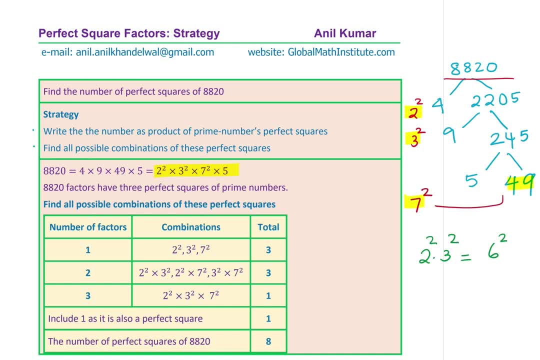 We need to find the combination of these right. So next step is to find their combinations. So, to find combinations, I made a table here, So we'll consider list of factors: perfect square factors, 1 by 1, and then 2 at a time. 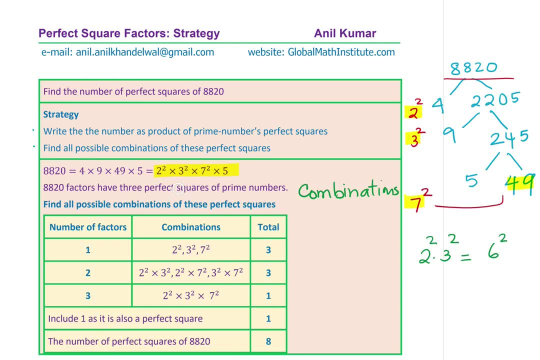 then 3 at a time. Well, we have 3.. So we can make combinations of 1,, 2, and 3.. So if I take 1 at a time, then I get 2 squared or 3 squared or 7 squared. 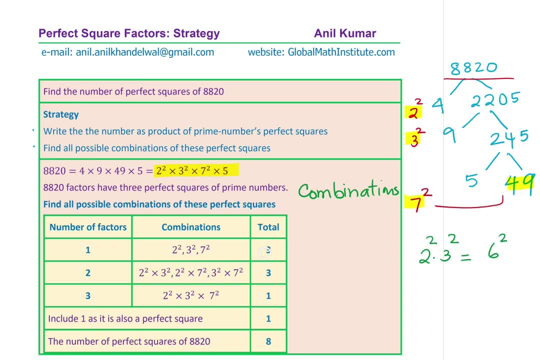 That means I have 3 perfect square factors of the number 8820.. When taking 1 at a time, Now I can take a combination. So if I take a combination, in that case 2 squared times 3 squared. 2 squared times 7 squared. 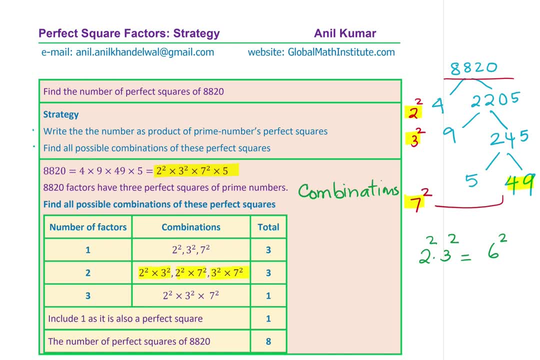 2 squared, 3 squared times, 7 squared are all the possible combination. We get 3 in all, in this case also, But we can take all 3 of them together. That gives us 1.. Remember, 1 is always a perfect square factor of any number, right? 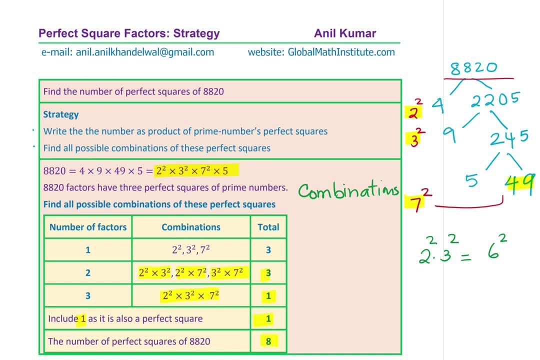 So 1.. 1 has to be included. Adding them all, we get 8. And therefore we can write our answer that the total number of perfect squares of 8820 is 8.. Correct, So that is how we can solve this question. 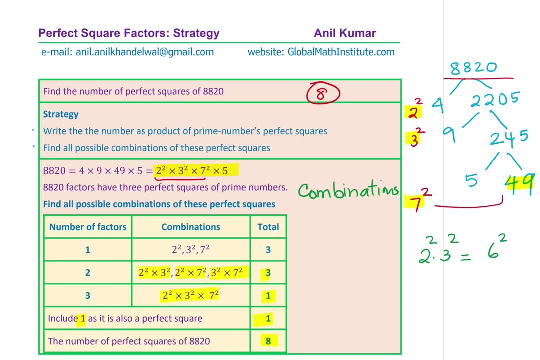 Well, there is a shortcut also, Once we get 3 factors. in that case we could actually get the answer 8, as 2 to the power of 3 is 8, right, So constant Combination. This is from the combination formula. 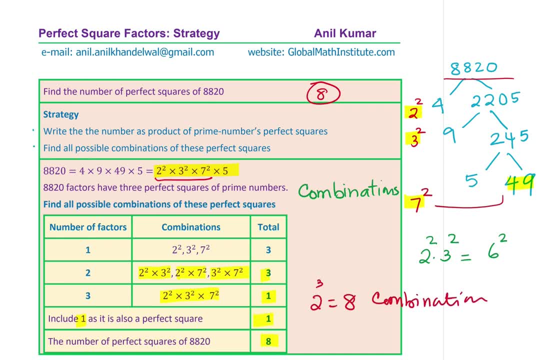 So combination with distinct numbers, right. So all the 3 which are for us 2 squared, 3 squared and 7 squared are distinct, right, They are not repeated. And if that is the case, in that case, 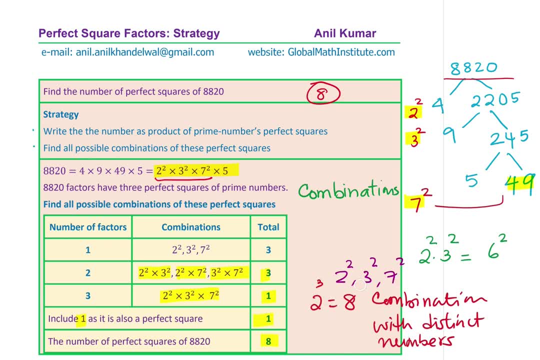 we get total number of combinations as 2 to the power of 3.. There are 3 numbers combination we are looking into. Well, some students may understand this part. However, the table form which I have discussed with you is absolutely clear. 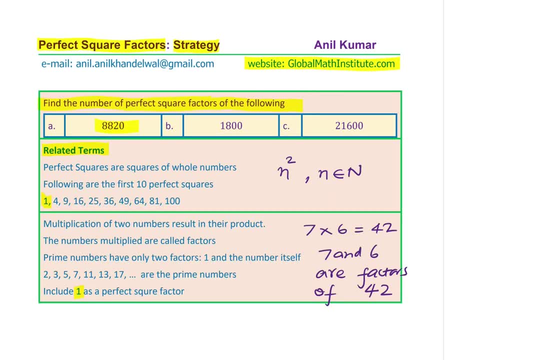 Now, with that in mind, what I would like you to do is- we have already answered this and we get 8 as our answer- I would like you to work on 1800, right? So 1800.. Begin with 1800,, correct. 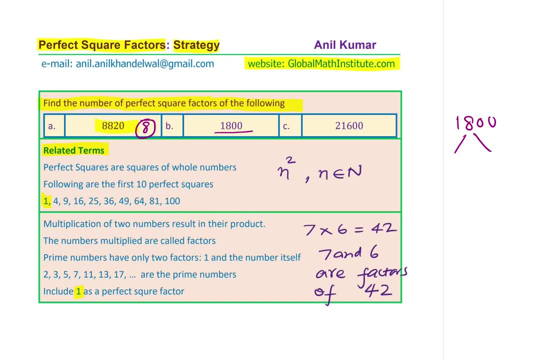 You can find. You can find the factors of 1800, then 18 is 9 times 2, right. So you could write 9 times 200, correct? So 200 is 100 times 2, right. 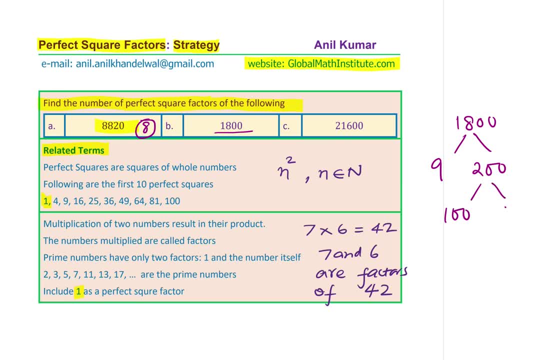 Which is a perfect square, correct 100 times 2, and 100 is 25 and 4.. So 100 is 25 and 4.. So that kind of gives you the combination of factors. You can write 9 as 3 squared. 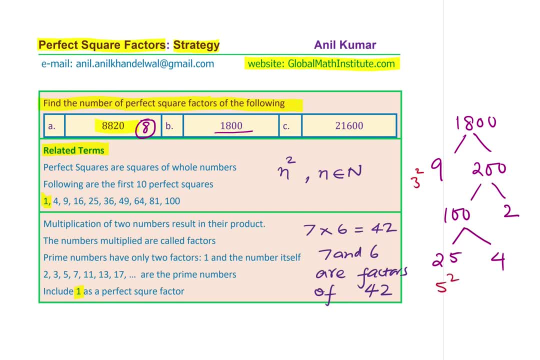 Correct, Correct. Correct: 25 as 5 squared and 4 as 2 squared. So you can now look into. there are 3 other factors and you should get answer as 8, correct? So I would like you to follow the strategy which we did for the first one and get the answer for the second correct. 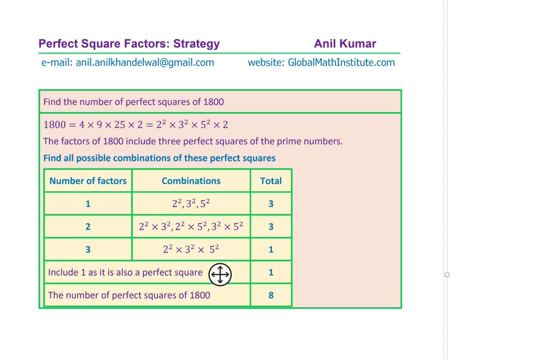 Now here is a quick solution for 1800.. We just did the same thing, So we find that 1800 can be written as 4 times 9 times 25 times 2.. Out of which 4,, 9, and 25 are perfect squares, and therefore we can write this as 2 squared times 3 squared 5 squared times 2.. 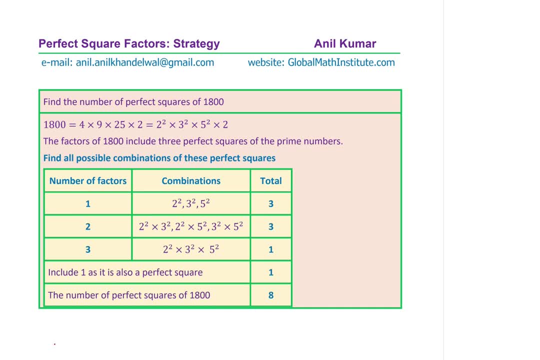 Now we'll once again take the number of factors- 1 at a time, 2 at a time, 3 at a time- and then we get these combinations which total to 8, and therefore 8 is our answer as the total number of perfect square factors of 1800.. 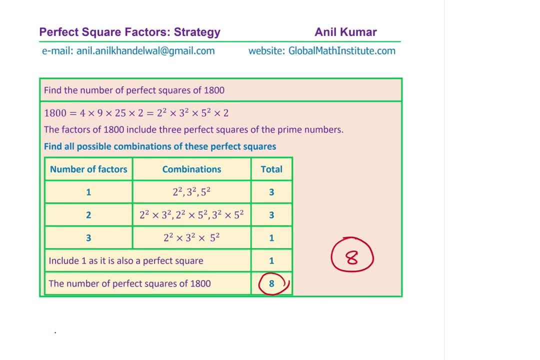 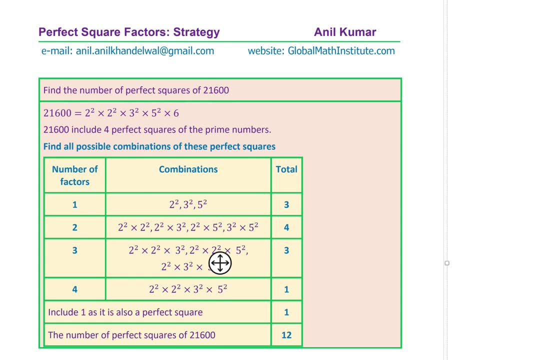 Is that clear to you? Perfect, Now let's take another one. Now, this is slightly tricky. Now we need to now find the prime factors of 21, 600,. right, So now we'll work on the number 21, 600.. 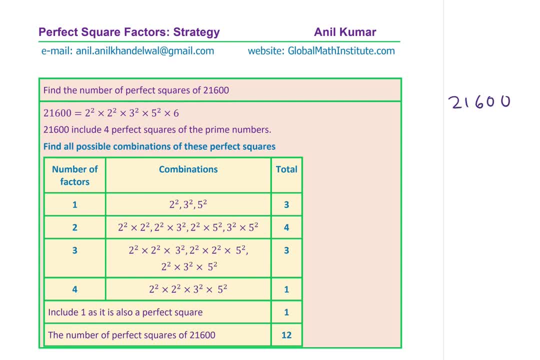 So let's write down the number 21,, 600.. How do we find these? Well, the steps are similar. 600 means 100 times right, So we get 216 times 100.. We could write this: 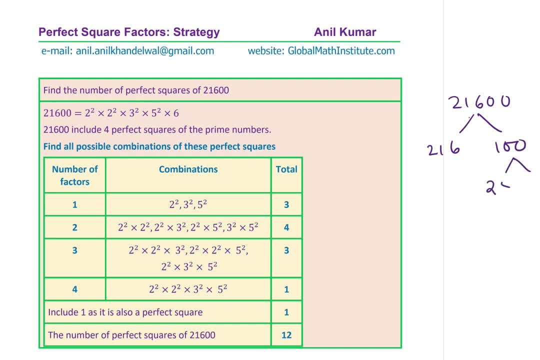 Perfect Faster, And 100 is 25 times 4, right, And 216 is 2 to the power of something correct. You get the idea right, So we can write this as some combinations of 2.. So let's first divide by 4 itself. 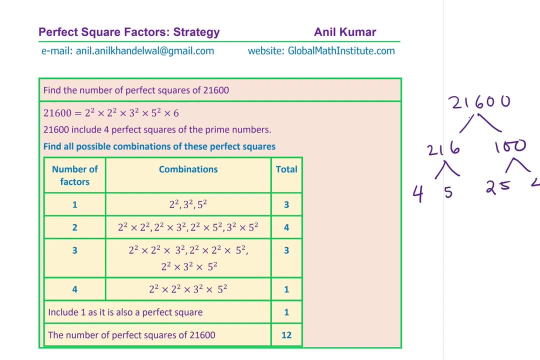 So when I divide by 4, I get 4 times 5, as 20 and 16 is 4,, correct, 54. And 54 gives me 9 times 6.. Correct. So these are the factors of 21,, 600.. 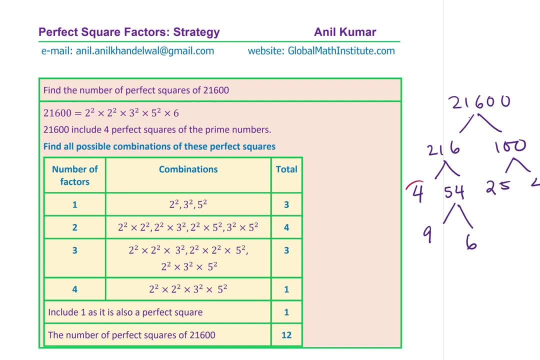 So that means we are looking for this as 2 squared, correct This as 3 squared, Perfect 25 as we're looking as 5 squared, And then again we have 2 squared, So we have twice. 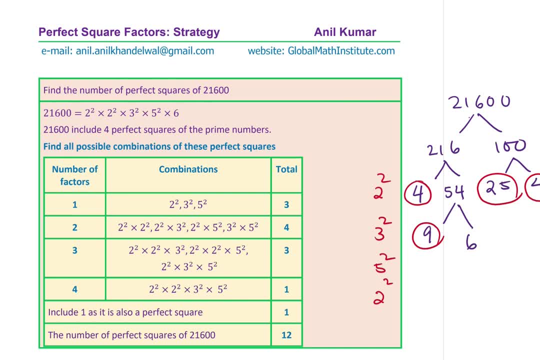 So the number 2 squared repeats. Do you see that? So that will give you the possible combinations And, of course, the number 6.. So I could write 21, 600 as product of 2 squared, 2 squared, 3 squared, 5 squared and 6.. 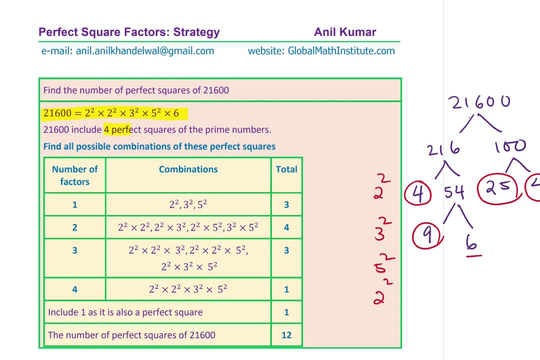 Now, in this case, you see that there are 4 perfect squares, 2, 2 being repeated. They're not distinct, right? So those who know the formula for combination, they can apply now the formula and get the answer. 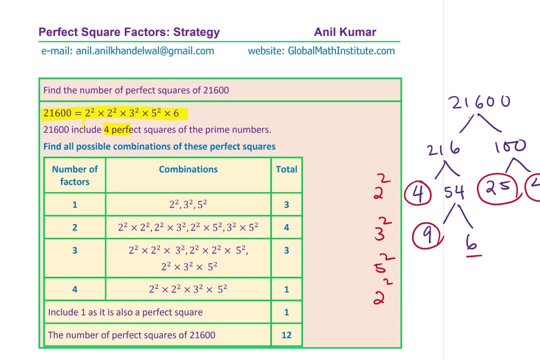 Perfect. Okay Now, if you don't know, then you make the table as we did earlier. Find all the combinations of these perfect squares, Taking 1 at a time, 2 at a time, 3 at a time and 4 at a time. 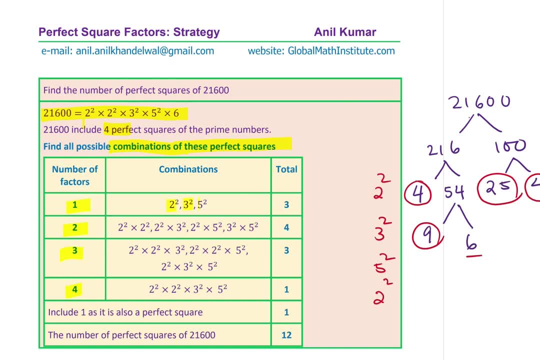 So well, if you take 1 at a time, you get 2,, 3, and 5 squares. So they're squares, So you get 3 in all, Taking 2 at a time. Remember, we have 2,, 2 squares, correct. 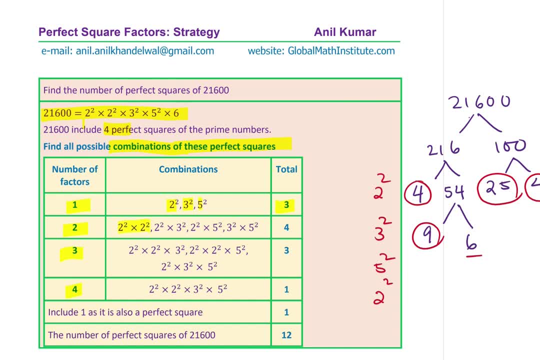 So, taking 2 at a time, we're going to have a combination: 2 squared times 2 squared, 2 squared times 3 squared, 2 squared times 5 squared And 3 squared times 5.. That gives us 4 combinations. 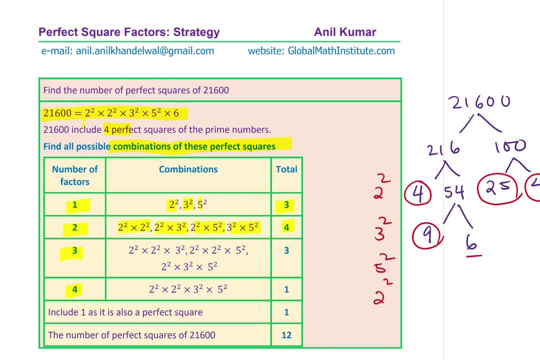 If you take 3 at a time, then we get 3 combinations: 2, 2, and 3.. Product of these squares And then 2 squared, 2 squared, 5 squared, And then with single, 2,, 3 and 5.. 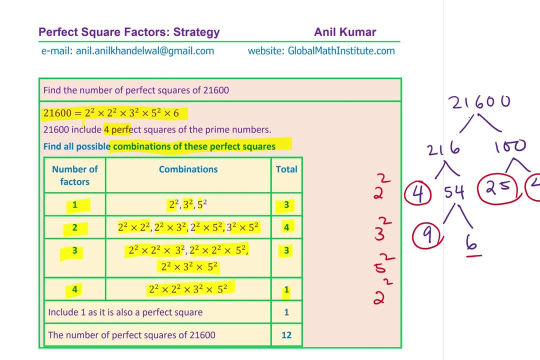 So we get 3 of these. Taking all 4 of them together gives me 1.. Remember, 1 is always a perfect square factor, And adding them, we get 12 as our answer: Perfect. So that is how we'll find the answer for this particular solution. 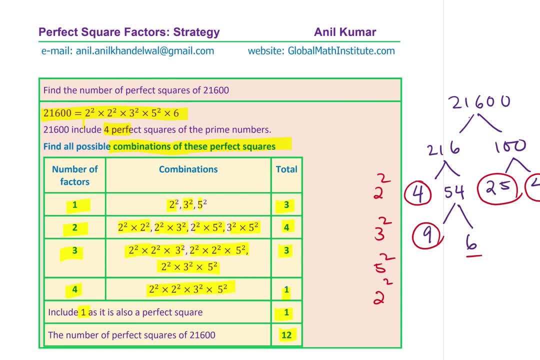 I hope that makes sense, right? Okay, So that is how you could do it. Those who know the combination, they can get to this result 12, very easily Using permutation and combination. Okay, But I hope with this you have understood. 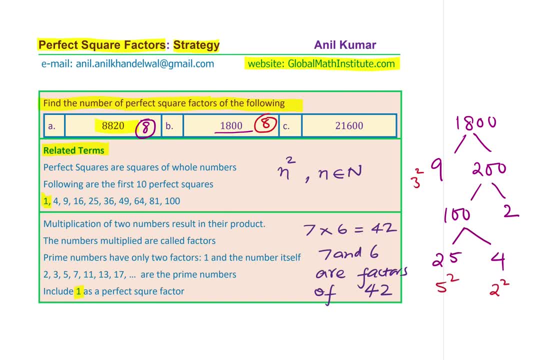 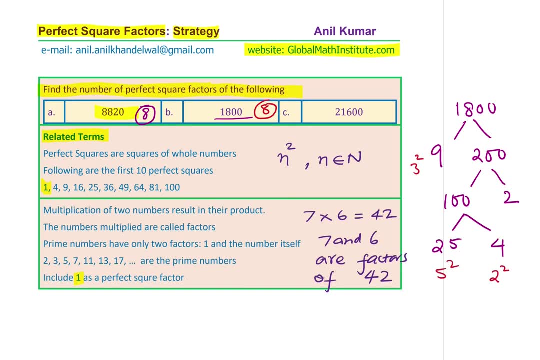 How do we find the perfect squares of any number, for that matter, Correct? So we get our combination for 21, 600 as 12. And that is how we should be doing it. Hope it makes sense. In case you want to learn from me, you can always send me an email on the address given here. 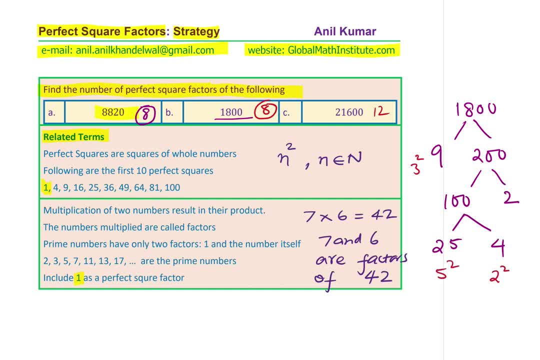 That should help. Thanks for your time and all the best.